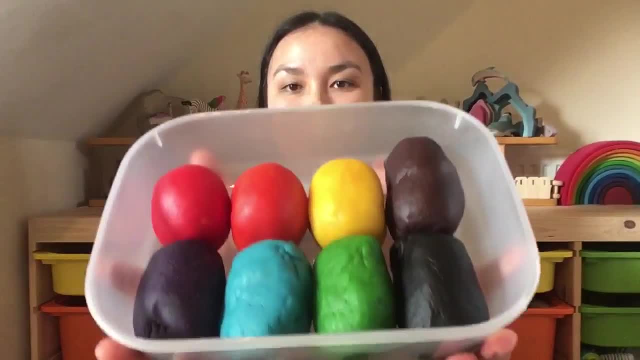 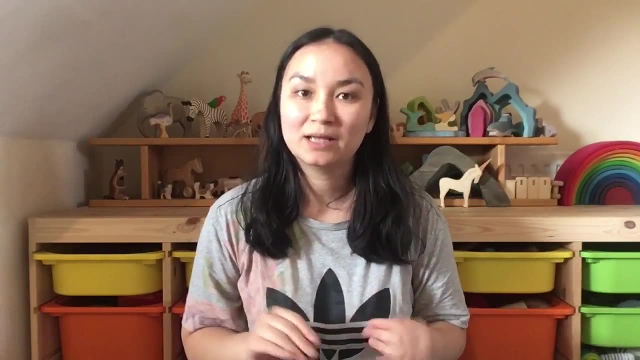 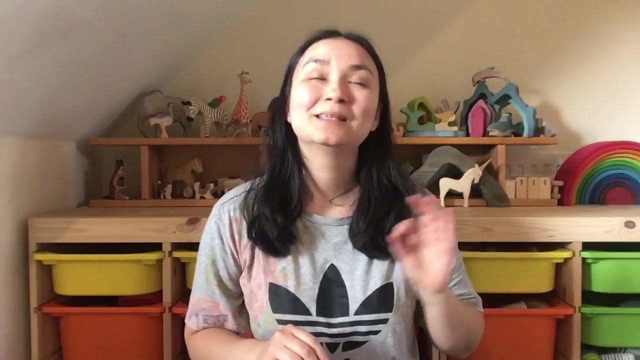 Hi guys, Today I wanted to share with you a recipe for some homemade play-doh that is super easy to make. It is non-toxic, so it's totally safe if your children still put things in their mouth, although they will probably spit it out, because it is salt-based. And the best part is it is super. 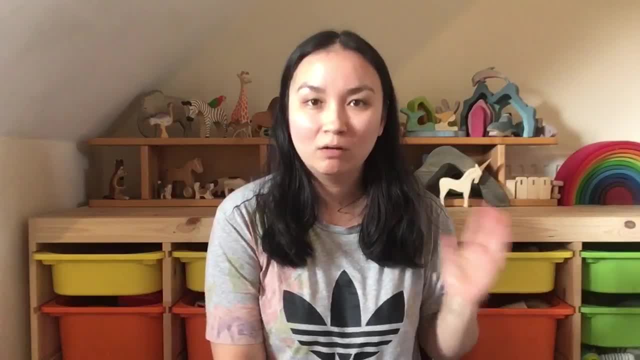 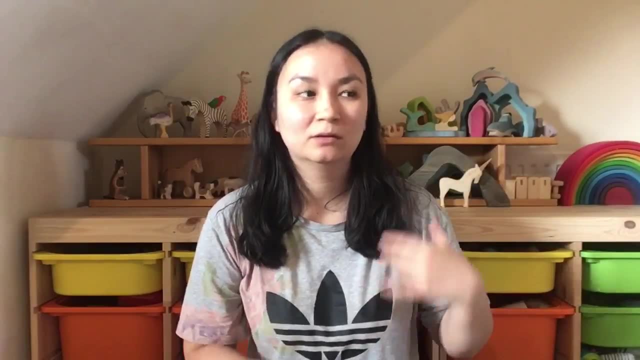 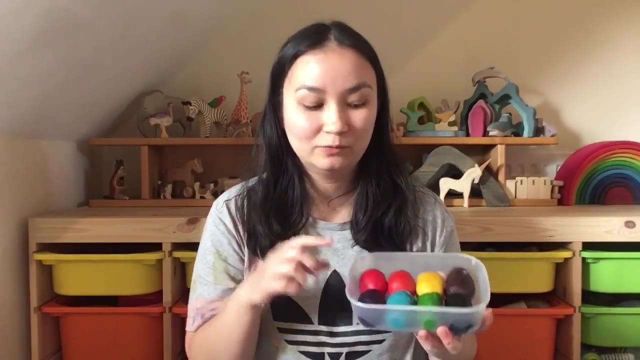 cheap to make. It's very economical, I'd say you can buy all of the ingredients for around three pounds, and I'm talking about an entire bag of flour, an entire thing of salt, an entire thing of oil. For the record, this was made from just the one batch that I made in this actual video. 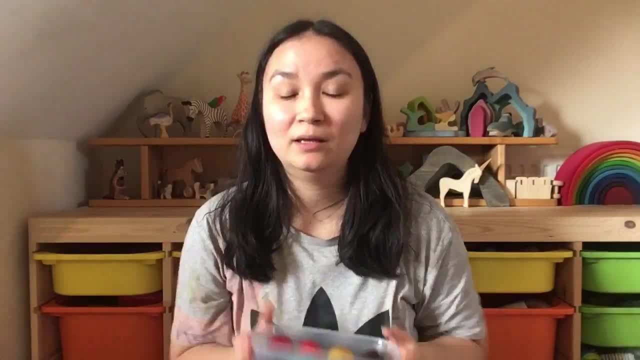 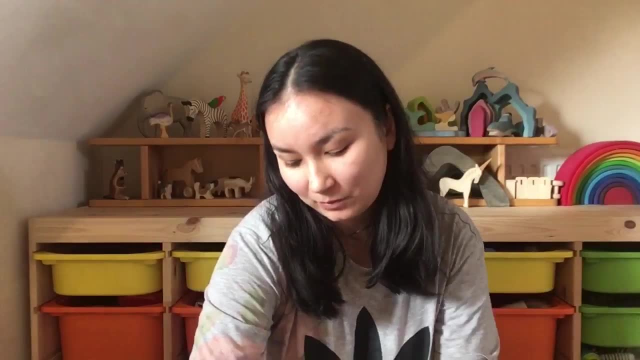 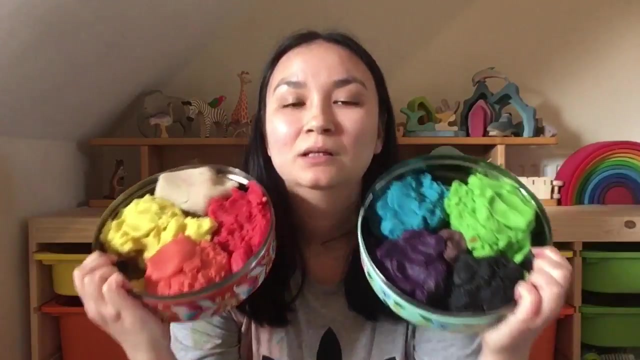 made all of these colors, So it is a very good sized batch and you can make quite a few colors from it. But I actually wanted to share this recipe with you guys, because I have this ginormous batch of play-doh that I made two and a half months ago- Two and a half months ago- and it is. 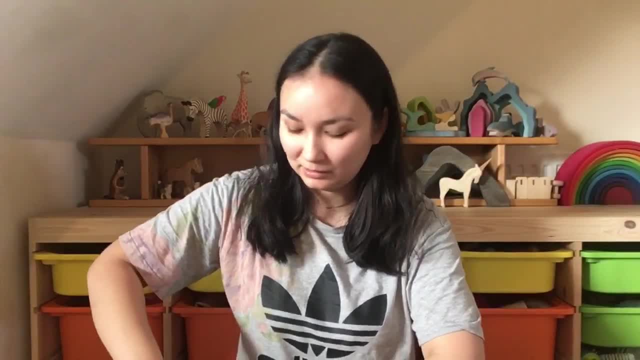 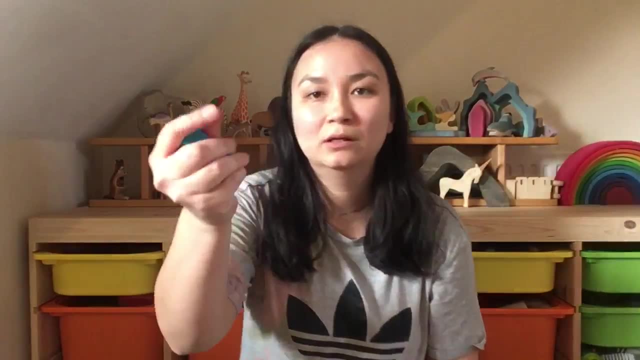 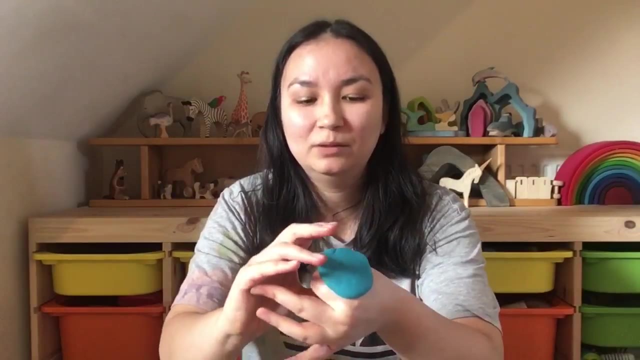 still going strong. My daughter has played with it nearly daily. It's often left out for an hour or two at a time without being covered, and it's still soft and pliable. It's very easy to work with, but it holds its shape when you mold it. It's just a really, really great recipe and I highly recommend. 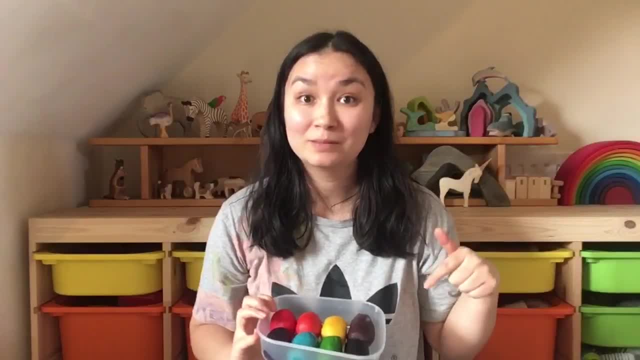 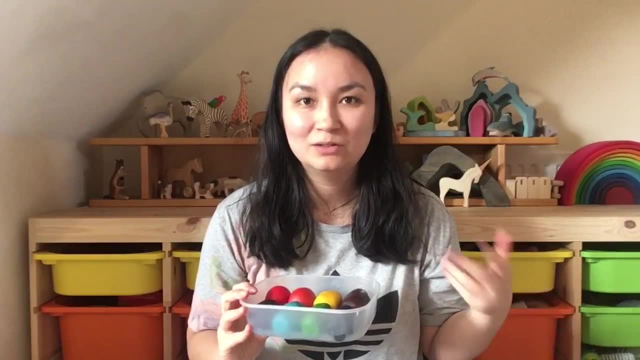 you try it. If you do try it, please let me know in the comments down below what you think of it. I'd love to hear your thoughts on it and I'll see you in the next video. Bye your input and let me know what your favorite things to make with play-doh are, because my 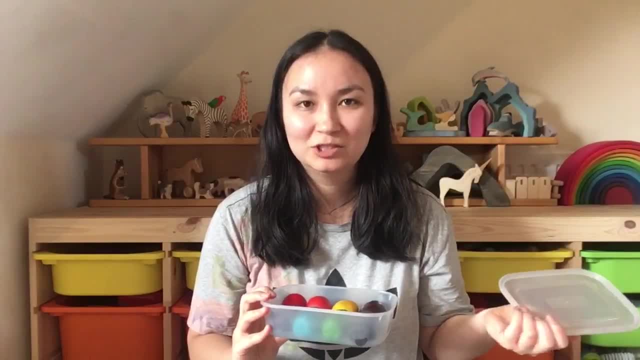 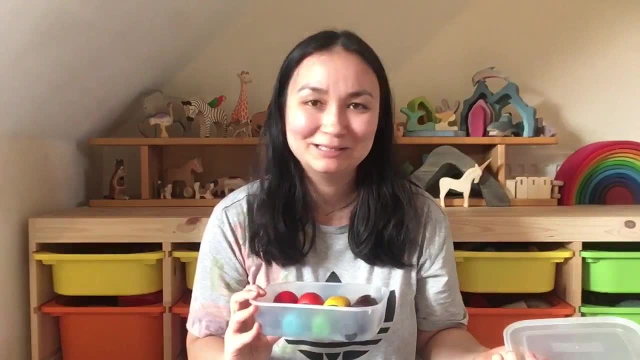 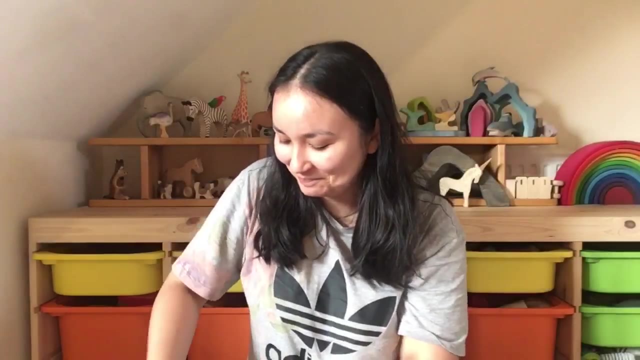 daughters are. basically, she likes to make fruit. she asks me to do all sorts of fruits with her. um, she knows how to roll out very simple structures like carrots and green peas, but i'd love ideas for other things to make with her. um, yeah, so i will see you guys for my next. 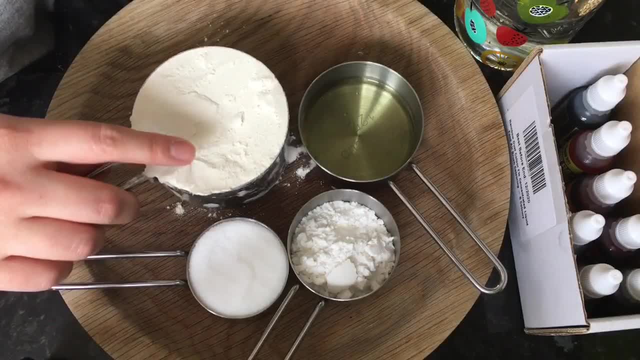 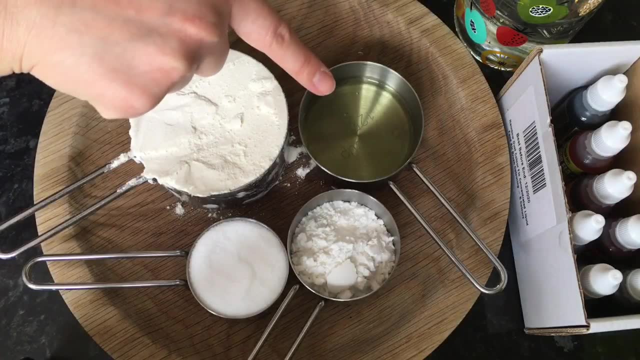 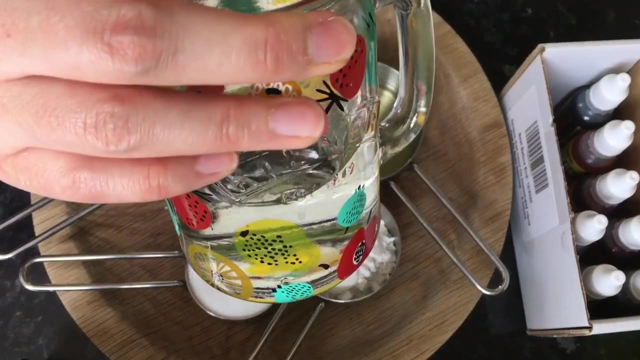 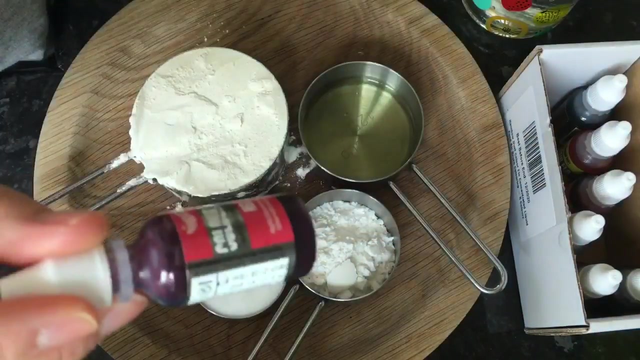 video. the ingredients are one cup of flour, a quarter of a cup of salt, two tablespoons cream of tartar, two tablespoons of any type of oil- but i am using vegetable oil just because it is the cheapest- and then a cup of water, and you want the water to be cold and also, at the end, you're going to want some type of food coloring. you can also. 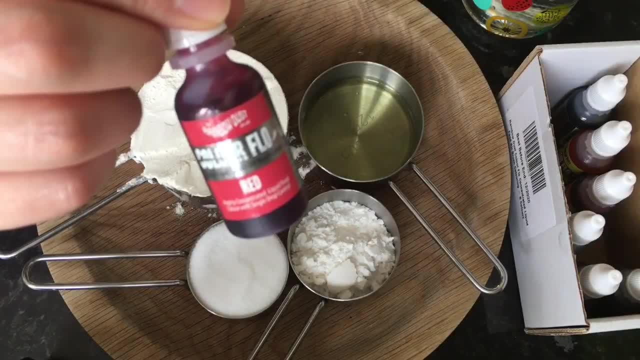 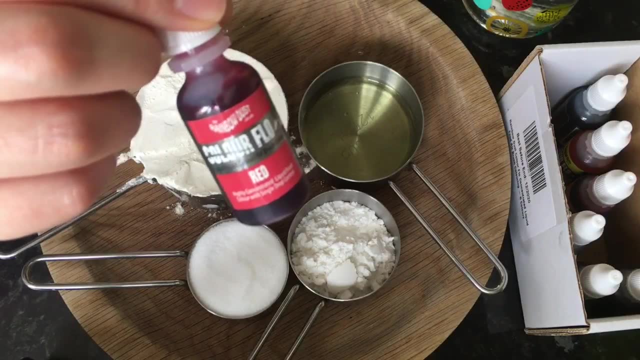 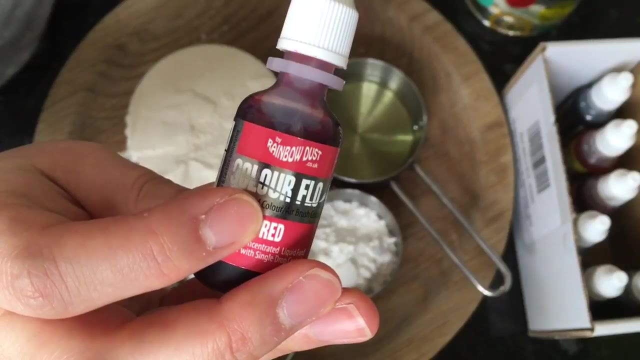 use like food powders that have colors to them, like strong pigments such as spirulina for green, beetroot powder for a red. you could use acai powder for a purple. um, and i do want to mention, for people who don't know or aren't aware, that normal food coloring generally is not vegan. 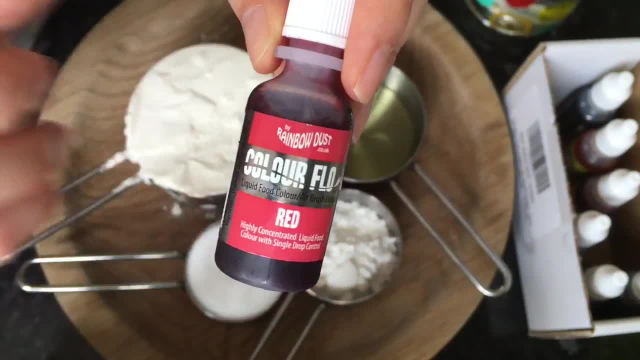 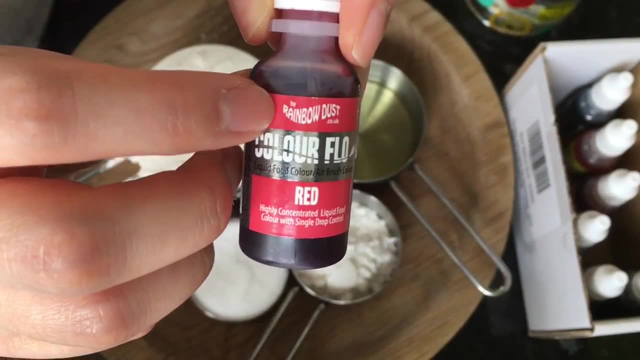 especially colors like reds and purples, or any color that uses red to make it. um, and this brand. i just found them on amazon. i just did a search for vegan food coloring. um, and this brand actually states that all of their food colorings are vegan friendly. so, yeah, i just wanted to share that with you. 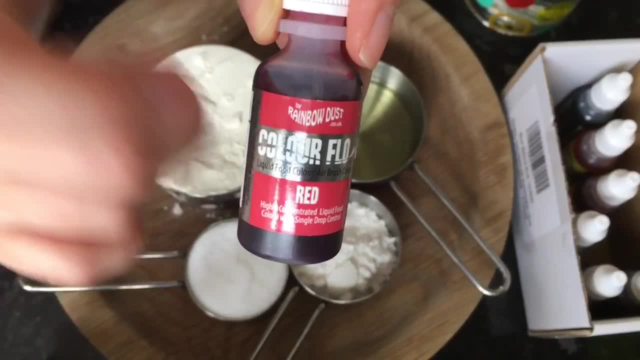 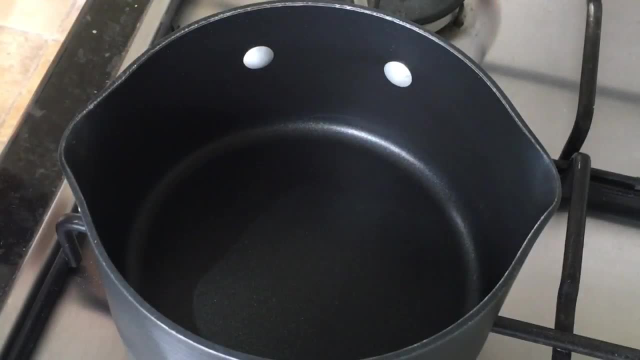 and i wanted to put that out there in case you were unaware, because i think that's good to know. so let's go straight into how we make this. okay, so making this is actually incredibly easy. that noise in the background is just the gas burner, but literally you put everything into the pan. 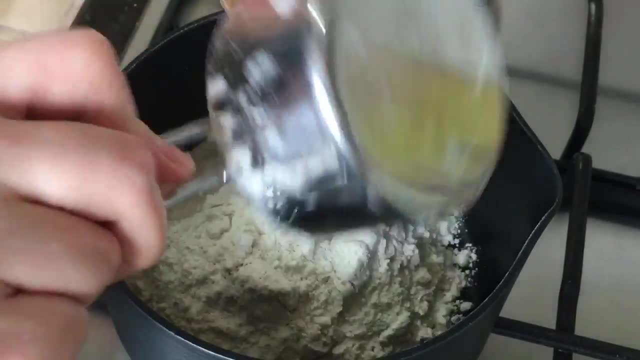 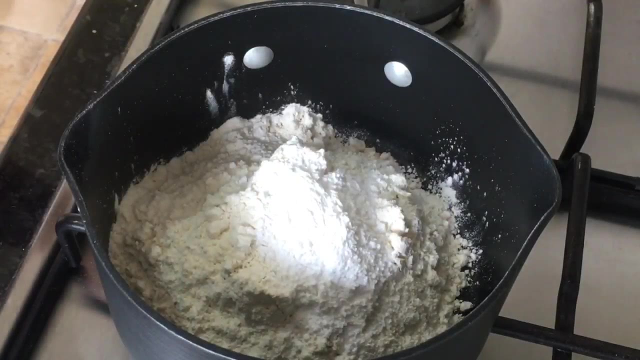 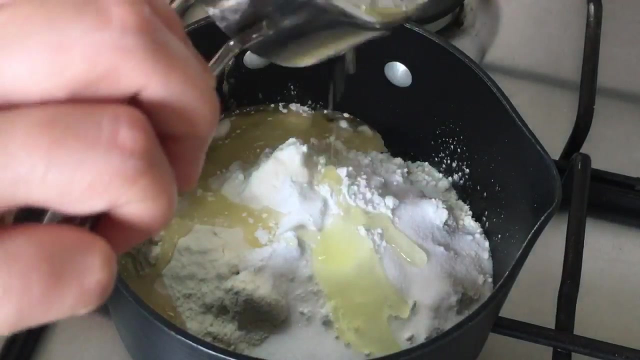 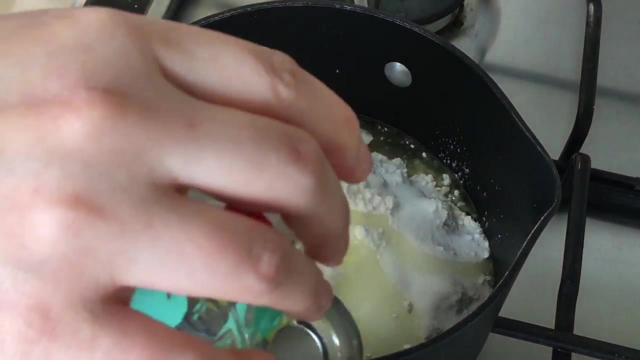 my flour is stuck. you just put everything into the pan at once, you don't have to do it in any specific order or anything. um yep, so that is the cream of tartar in the flour, i've got the salt oil and, lastly, the water. 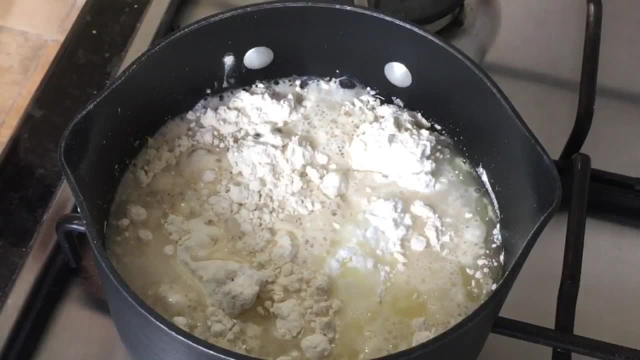 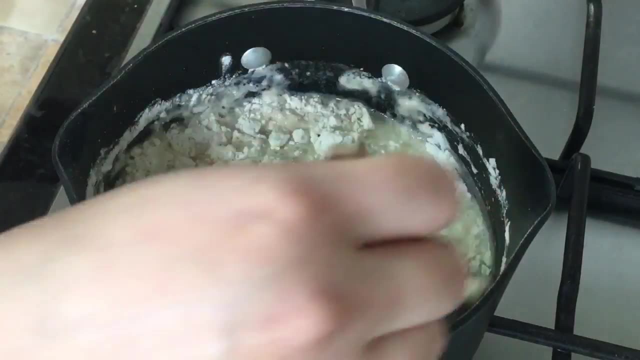 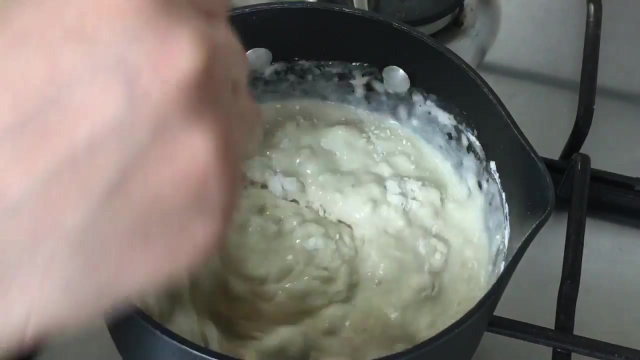 and you just want to keep stirring this over a low heat and basically this is going to be a couple minutes of stirring. so i am going to go ahead and speed this up until we're at a point that is better, better, better, better to talk about, um, but basically we're going to just keep stirring it until it forms a ball. 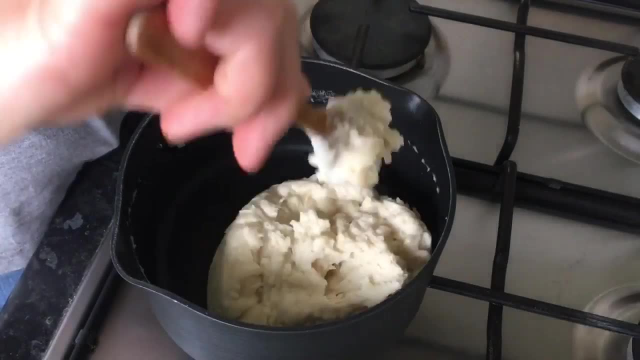 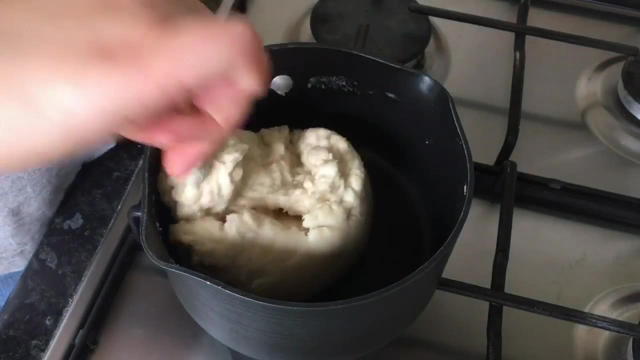 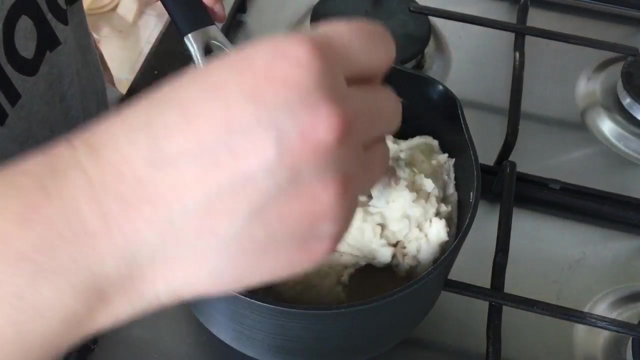 all right. so that literally took about one to two minutes of stirring to get to this point. um, so now i've got a lump that i can't really stir too much anymore. um, because it's just a lump. but i am going to keep this on the heat for a little bit longer because you really want some of this moisture to. 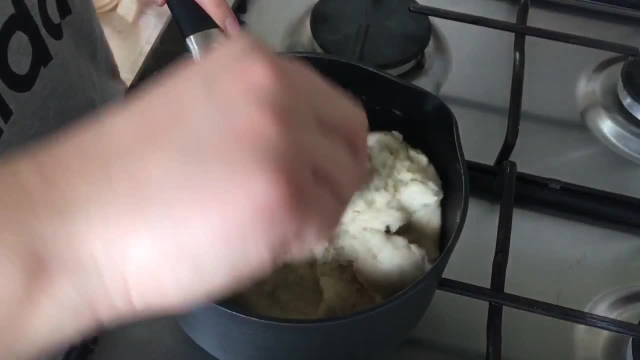 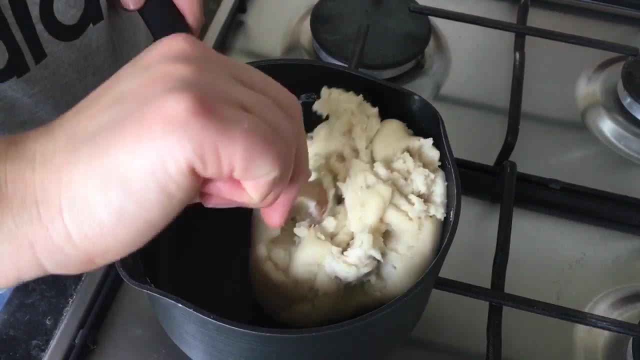 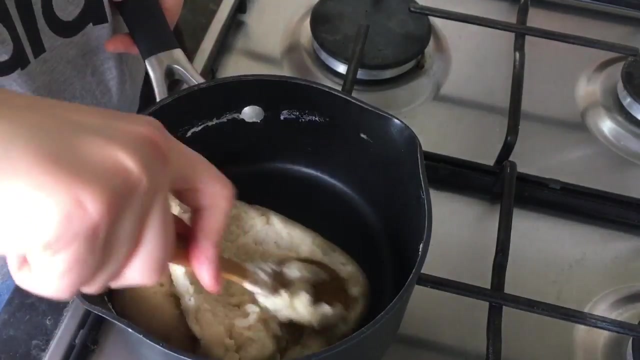 come out of the dough because um, otherwise your dough ends up a little bit too sticky and harder to work with. so this is obviously a little bit harder to work with at this point, but just keep working with it and trying to. um, basically my goal right now is just to keep um moving it around. 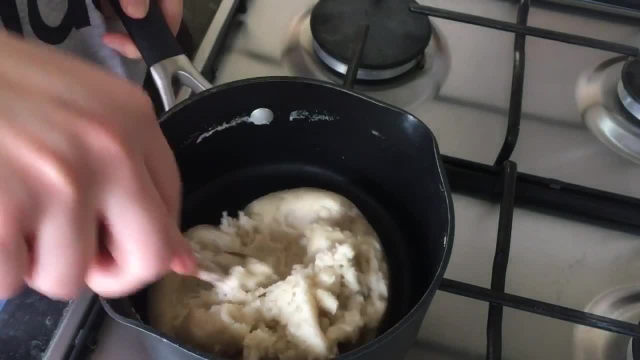 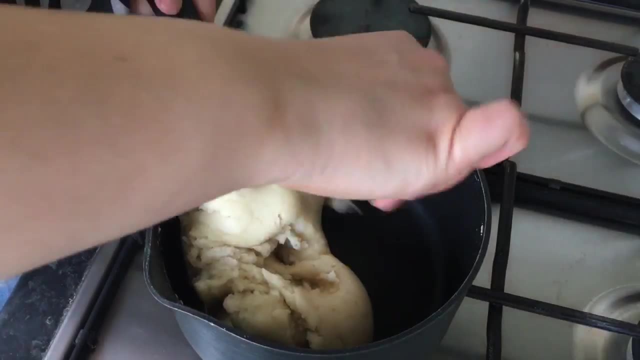 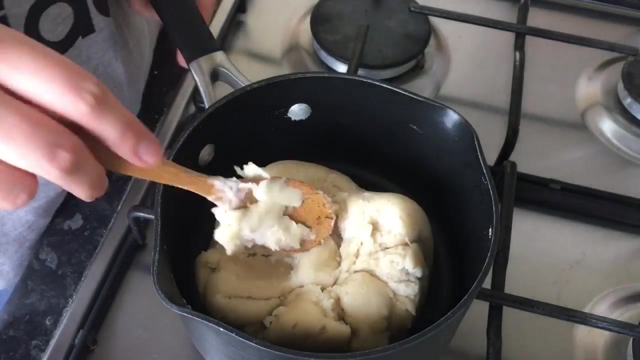 with the spoon and exposing new areas of the dough so that it doesn't stick to the bottom of the bowl. as to the air, so that a bit of the water in it can evaporate out, um, and then also trying to fold over from the bottom so that new parts of it are exposed to the heat as well. um, hopefully that all. 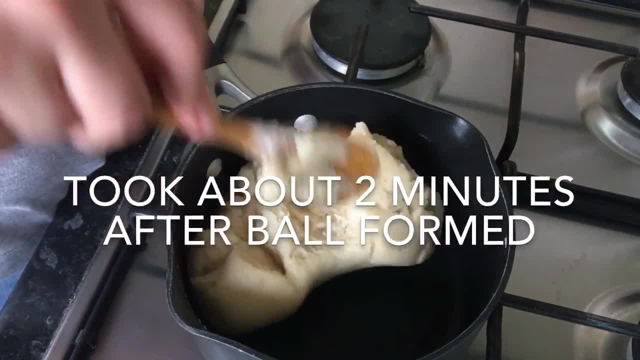 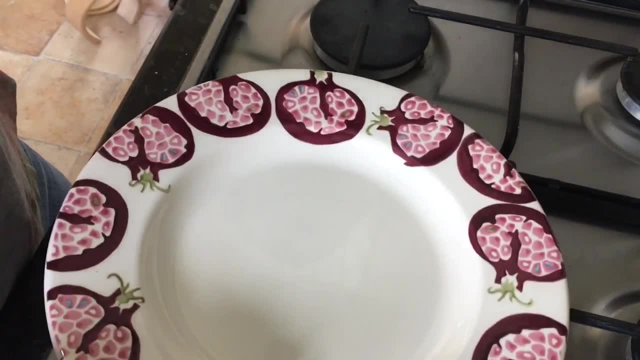 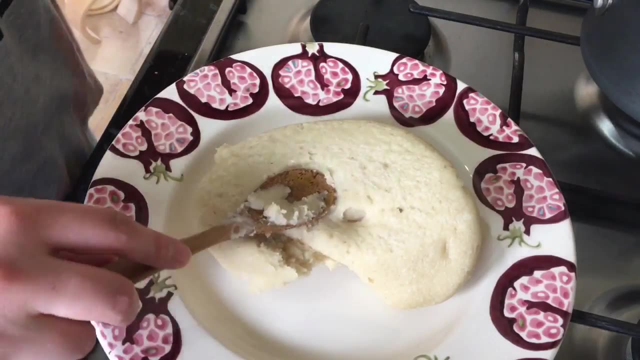 makes sense to you guys. so at this point i would say that this is done. so what i like to do- um, just to speed things up a little bit for me is: i'm going to go ahead and stir this up a little bit. i like to put it out onto a plate and then i like to just kind of, um, flatten it out quite a bit. 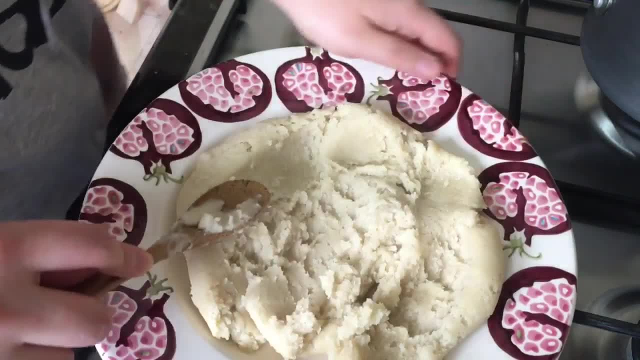 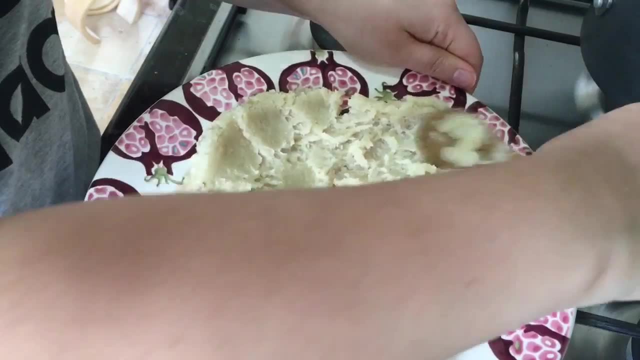 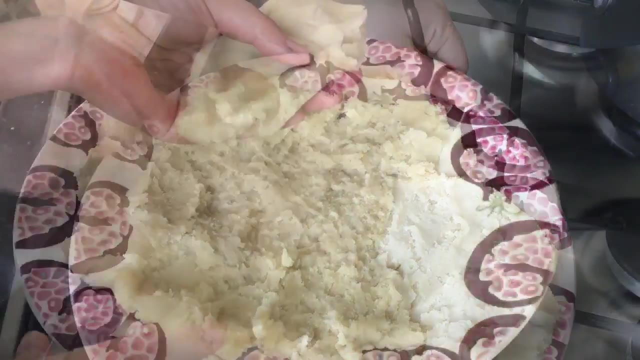 so that it can cool down faster. this is like optional. this is just because i have like barely any patience, um, but yeah, this will just um create more surface area, so it will cool down faster. i'm being repetitive, sorry guys. okay, so this has been cooling down for. 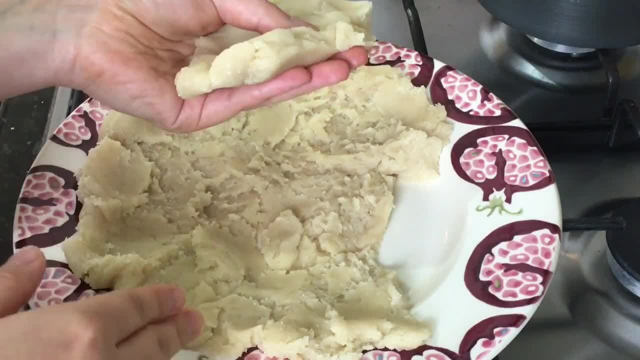 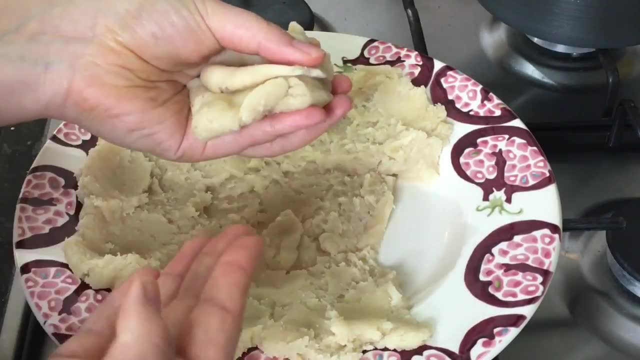 about 20 minutes, but really you can work with it for a little bit longer, and then i'm going to let it cool down completely and work with this at any point. um, basically, as soon as it is cool enough for you to handle it, you can work with it and you can let it cool down completely and work. 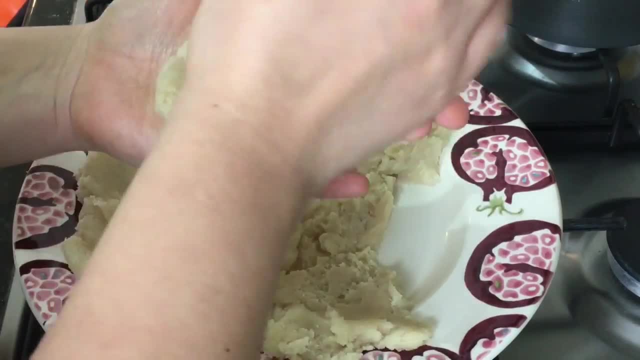 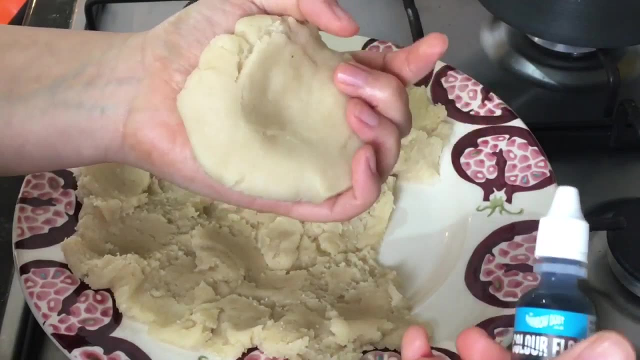 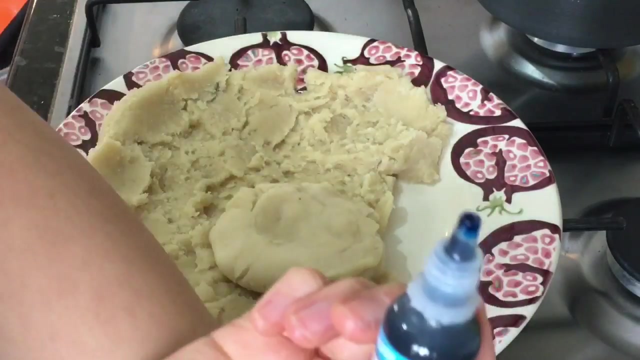 with it like days later. so, um, what's nice about this play-doh is that it is so soft and easy to work with that, if you add food coloring to it after mixing the dough, um, it integrates very easily and smoothly, whereas, um, some restaurants will do it like this and i'm going to show you. 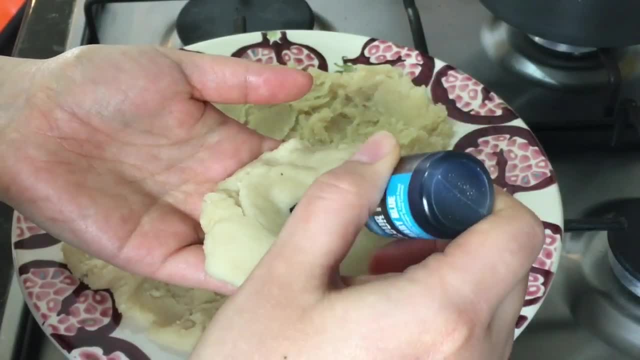 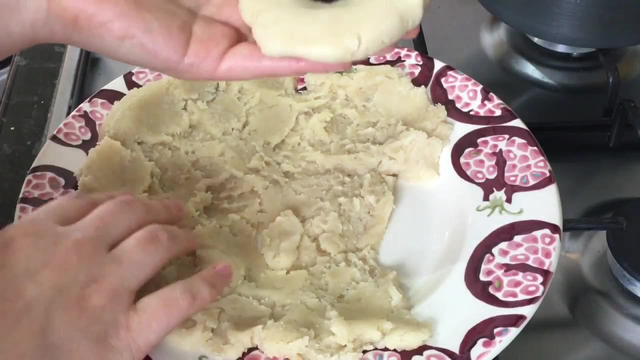 how to do it and what that looks like in a bit. that's super 있어요 on you. um, but nuclear creates this medium six to plug stick lim tiet. yeah, i've got a little bit here. this piece is just just it. it i kind of I'm just gonna zest it, it out and i'm just gonna 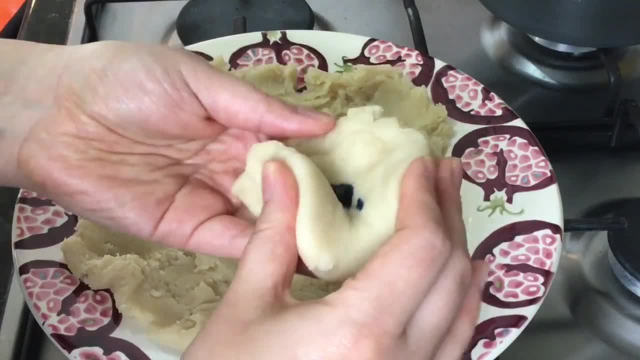 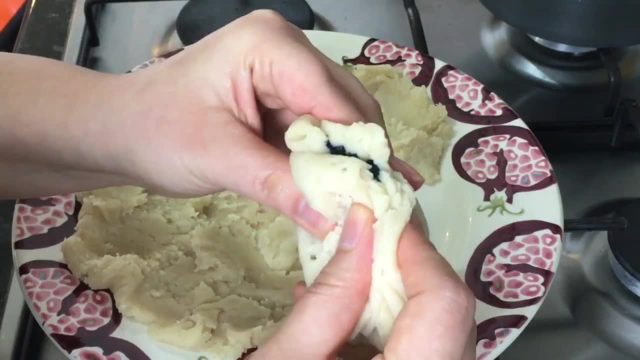 knead it, and then i'm going to process the dough to the form they call it for. i'm gonna knead it in between. um, actually, since i'm getting really surprised at how Riley is doing with different recipes, i think i forgot to just add a little bit at a time to make it. 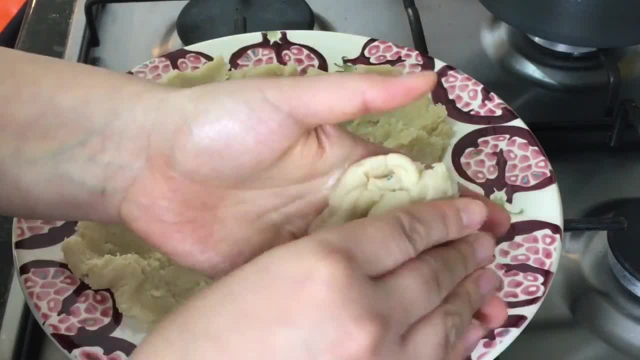 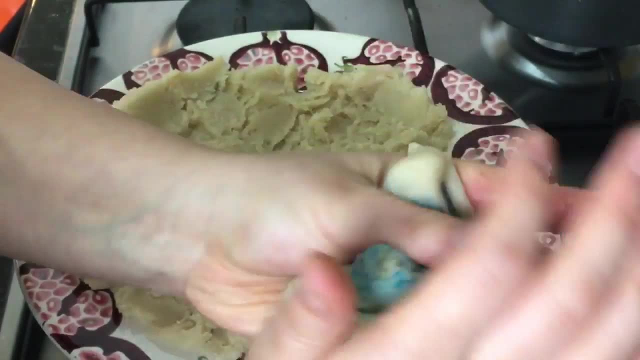 like just really, you can just kneading it, and this is another recipe i make. if you have vegetable color comes up, you can add more drops, but you can see that it starts working throughout the dough fairly quickly. so I'm just gonna keep kneading this. so I